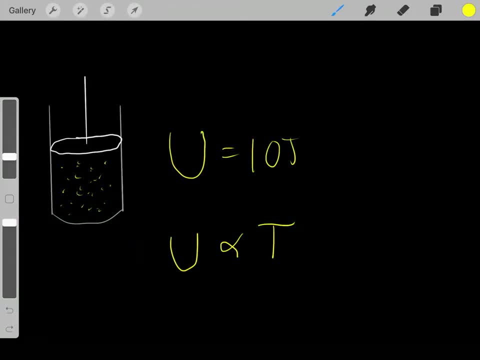 temperature of the system. They're proportional. So therefore you might wonder: how do we raise the internal energy of the system? And there are two ways you can raise the internal energy of the system. One way is by adding heat is by adding heat to the system And the symbol we use for heat. 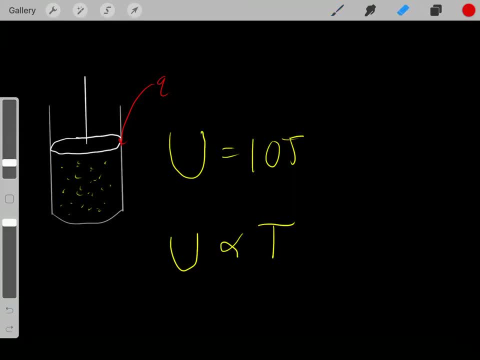 is Q. So let's say, originally the system had 10 joules of internal energy, But then we add in 5 joules of heat energy. Now how much internal energy does the system have? Well, now the system would have 15. 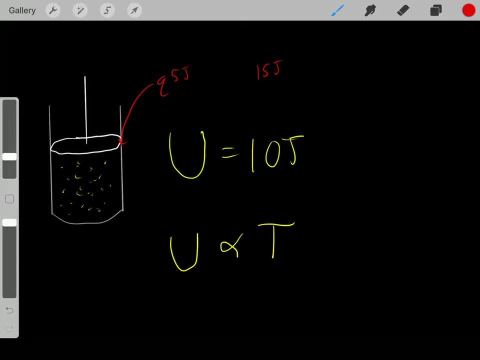 joules of internal energy. And not just that: we know it has more internal energy. So we know it has more internal energy. So therefore the temperature must have increased, And that makes sense. We add heat, we raise the internal energy and we raise the temperature. That makes sense. 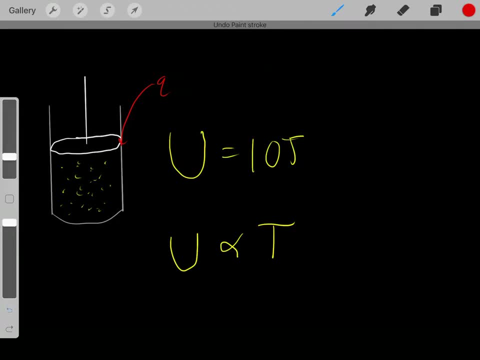 Adding heat raises the temperature. However, there are other ways we can raise the internal energy. Heat is just one of the ways. Another way we can raise the internal energy is by doing work on the system. If we do work on the system on this gas, if we compress this gas and we do some work on this gas, we can also raise the. 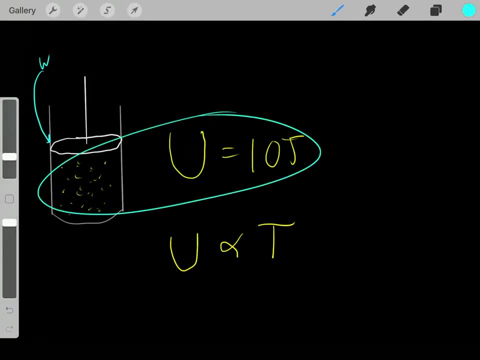 internal energy of this gas. Again, let's say that originally we had 10 joules of internal energy, But then we do 5 joules of work on this gas. Now the gas has 15 joules of internal energy, So therefore the internal energy has increased. 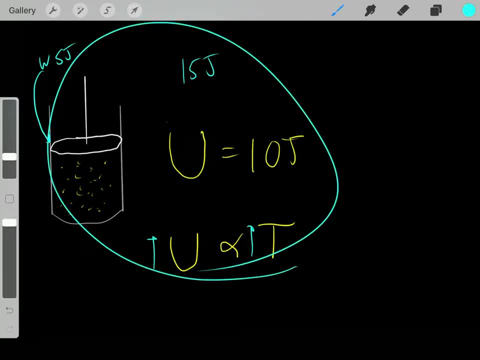 Now the temperature has increased And notice, this is not intuitive. Yeah, adding heat, raising the temperature, that makes sense. However, we can also do work on the system. If we do work on the system, that also raises the internal energy, That also raises the temperature, So we can do. 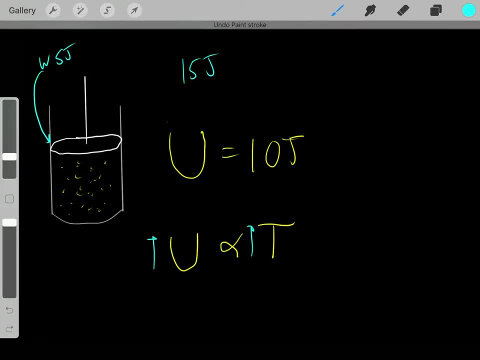 work. we can compress this gas and that would also raise the temperature. So again, that's not entirely intuitive, But again there are those two ways we can raise the internal energy. We can do heat, we can add heat or we can do work. And this is the essence of the first law of the law. 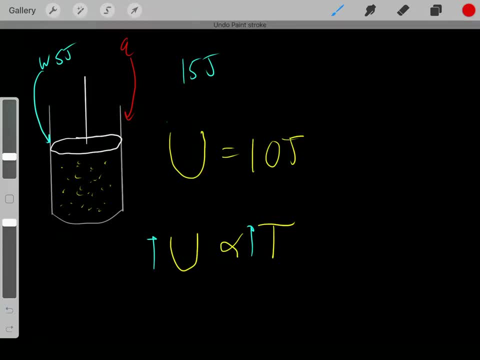 So we can do work. we can add heat or we can do work, And this is the essence of the first law of the law: The only way we can change internal energy is heat and work, Even though, in reality, if you were to, 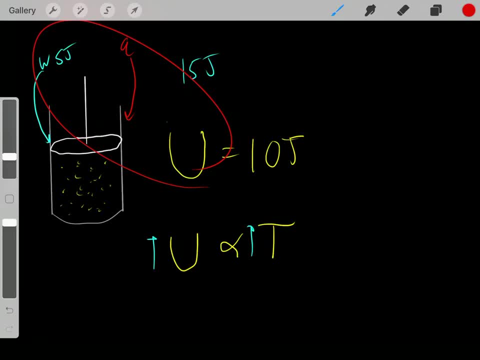 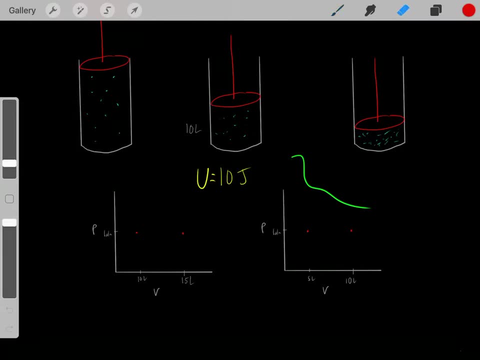 read a typical thermodynamics textbook, you would see that that's not true and it's a little more complex than that. But again, that's the basic principle. So, again, so, let's say so. let's do some examples. Let's say we have this system. Let's say we have this system And let's say it's. 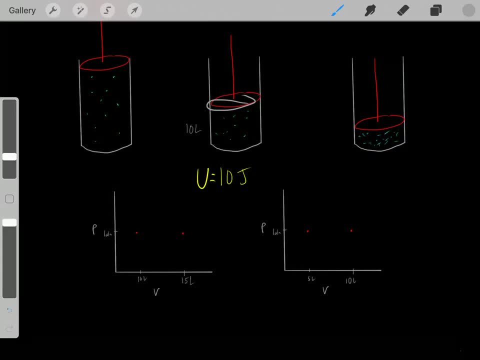 10 liters, And let's say so. there's 10 liters of volume in the system of these gas particles, And let's say it has 10 joules of internal energy. And let's say it has 10 joules of internal energy. 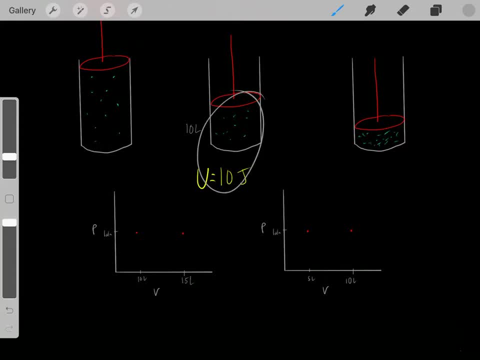 And let's say it has 10 joules of internal energy. Well, again, we said we can change the internal energy by either adding heat or doing work. So again, if we have 10 joules of internal energy and we add five joules of heat, then again, now the system would have 15 joules. 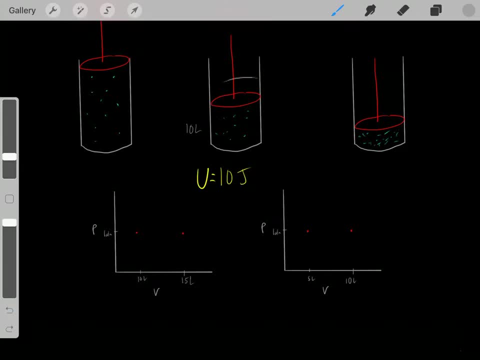 of internal energy and the temperature would increase. But we know we can also do work on the system. we can do work on the system and that will also increase the internal energy. So again, how do we do work on a system? Well, if you haven't taken physics, 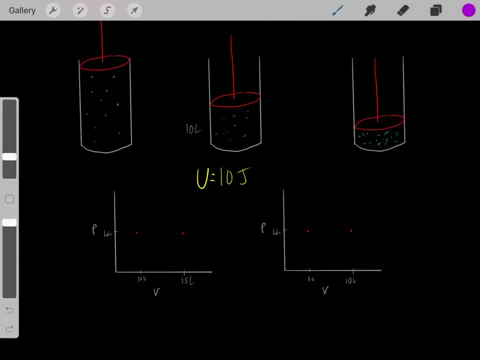 don't stress out about this too much, But essentially, what you can do is, whenever you have a system and you apply force over a distance, you're doing work. We know. we know a force times a distance equals the work done. So therefore, therefore, if we apply to, 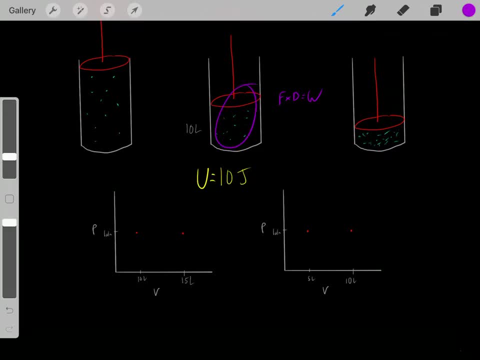 force on this gas over a distance, we did some work on this gas and we could do work on this gas. So, again, if we apply to force downward and therefore compressed this gas, we would do work on this gas And again, let's say we did five joules of work. 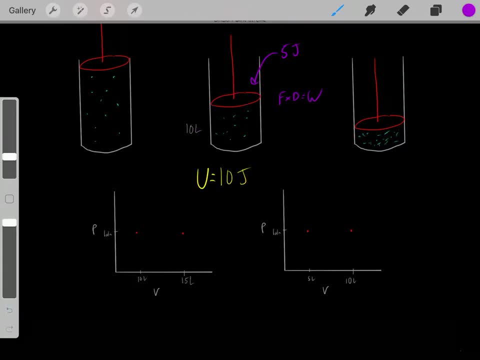 Let's say, originally we had 10 joules of internal energy, but then we did five joules of work. Now we know the system. now we know the system would have 15 joules of internal energy. And again we know we raise the internal energy, so we raise the temperature And again. so the key: 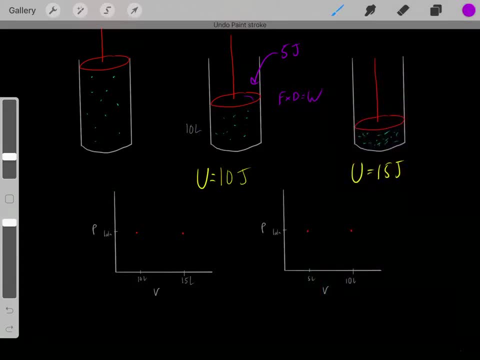 point is, whenever you compress a gas, whenever you're compressing a gas and you're compressing and the volume is decreasing, you're doing work on the gas Because, again, you had to apply force to compress this gas. We know there's pressure, so therefore, to compress this gas, you have to. 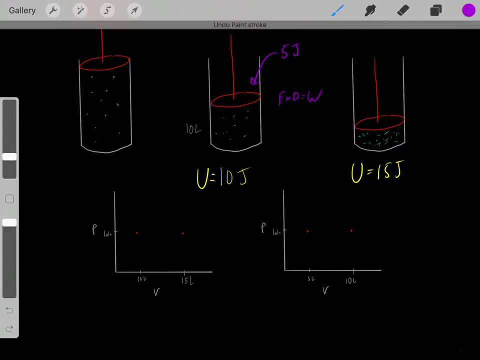 apply a force over a distance. So, therefore, when you compress gases, that's when you do work, that's when the system has gained internal energy. the internal energy increased when you compress a gas, And again it's because we're doing a force over a distance, But in reality, because this is, 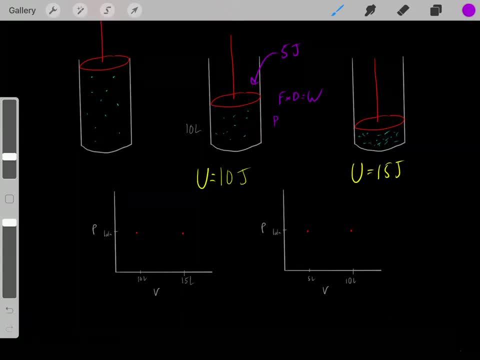 a 3D system. really, what we're doing is there's a pressure and we're changing the volume. So at a given pressure, we're changing the volume from this volume to this volume. So therefore we had a change in volume. We could change the volume from this volume to this volume, So therefore we had a 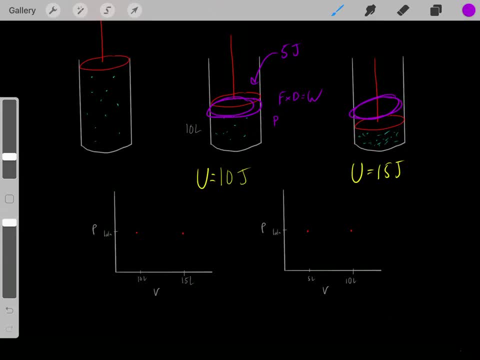 change in volume. We could see this much volume had changed. We could see this about this much volume had changed. So, therefore, what's important to note is, if you know the pressure of the system and you know the change in volume, you know what the change in volume was then, therefore, you can. 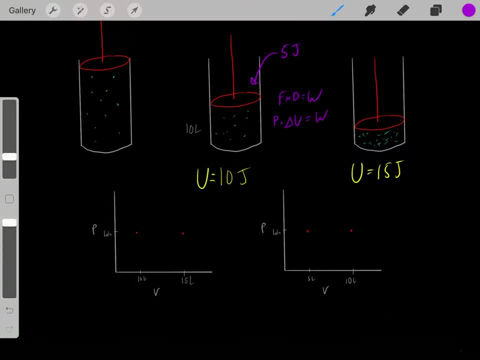 find out how much work you must have done. So again, so based on what the pressure was and based on what this volume was, this change in volume that we saw, we could calculate that and we could see how much work we had done And we said we did five joules of work. So the key point, 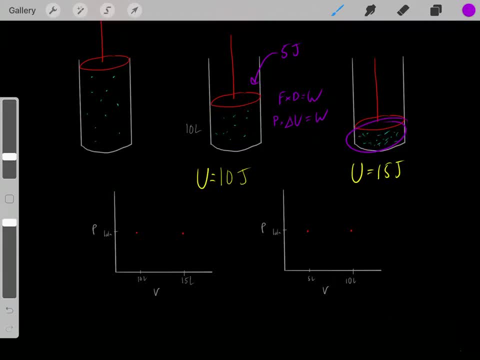 is when you compress a gas, you're doing work on the gas, and the gas raises its internal energy. However, what if we went in the opposite direction? What if we decompressed a gas? Well, remember, when we compress a gas, the gas raises its internal energy. So, when we decompress, 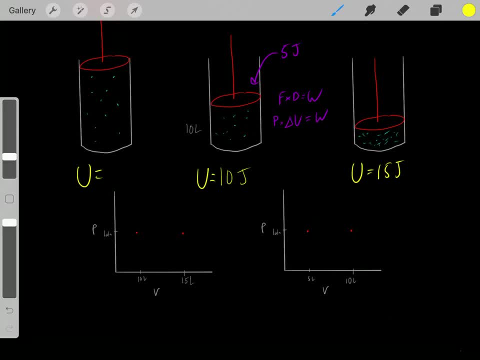 a gas, it loses some internal energy. So now its internal energy would maybe be five joules and it lost internal energy Because, again before, in this situation, we were doing a force on the gas, we were doing work on the gas. 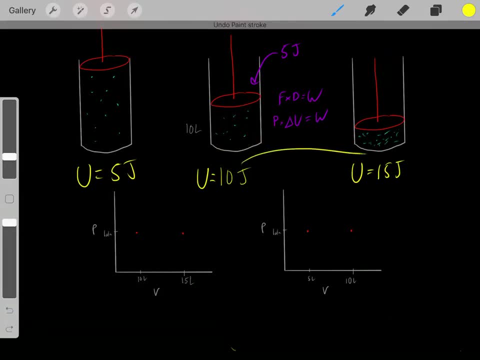 Applying a force over a distance. So we were doing work on the gas, so it gained energy. However, in this situation, the gas lost energy. Essentially, what happened was the gas was now doing work on the atmosphere. The gas was decompressing. It was decompressing, So 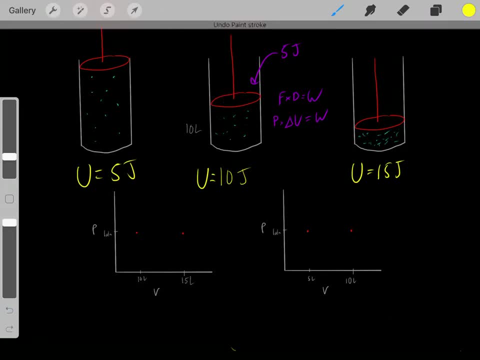 therefore applying a force upward, doing a force on the atmosphere. So it did work on the atmosphere. So therefore it lost that energy and the atmosphere gained that energy. So now the system lost internal energy And therefore we would see the temperature would decrease. 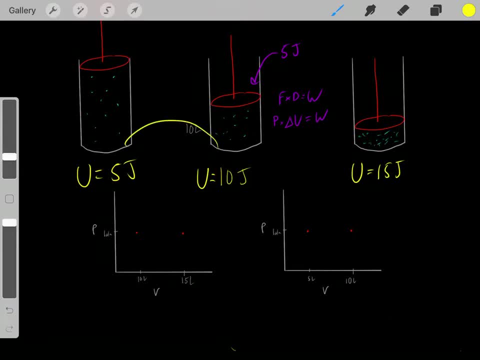 And again, we were doing work on the gas, so it gained energy, So we were doing work on the atmosphere. So again, how do we find out how much internal energy it lost? Well, again, if we know the pressure times, the change in volume, what this change in volume was, then we can determine how. 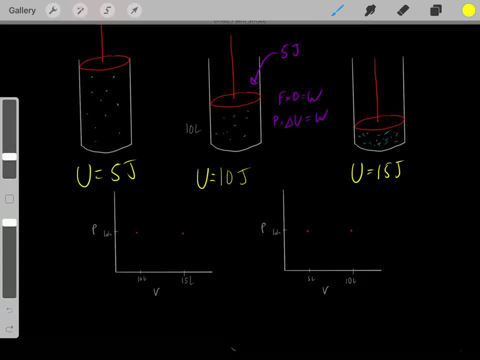 much work it lost and how much energy it lost. And again, in these situations we're assuming that the pressure was constant, which kind of simplifies the math. But now let's talk about these PV diagrams. So these are common diagrams. you'll see in physics and chemistry classes. 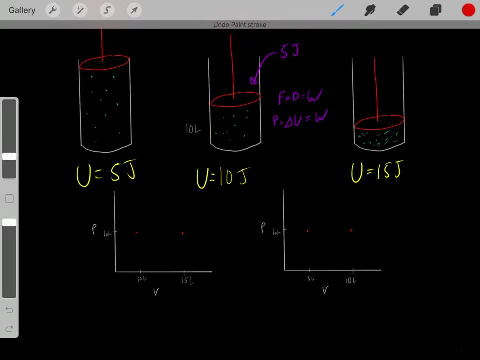 So let's draw a PV diagram that represents this situation where we did work on the gas. Well, in these PV diagrams this axis represents the pressure and this axis represents the volume. So again, we said originally we had 10 liters. So let's say we had a certain pressure. Let's say we 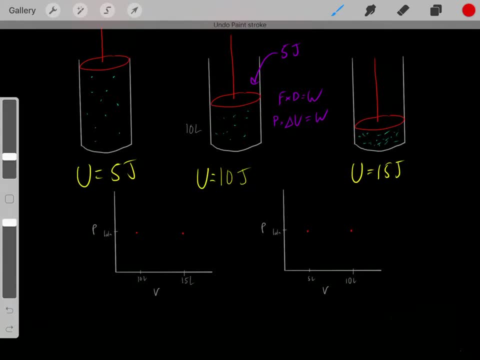 were at one atmosphere pressure and we had a certain volume at 10 liters. So therefore this original situation would be represented by this dot. But then we did work on the system. We did work and we compressed this gas, making its volume decreasing. We decreased its volume. 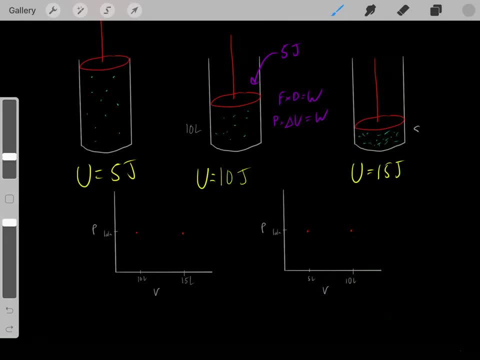 so now its volume decreased to, let's say, 5 liters. So therefore we know we did work on the system. So now it's: this system has 5 liters of volume. So now we would be at this situation where the volume is at 5 liters. So this graph- 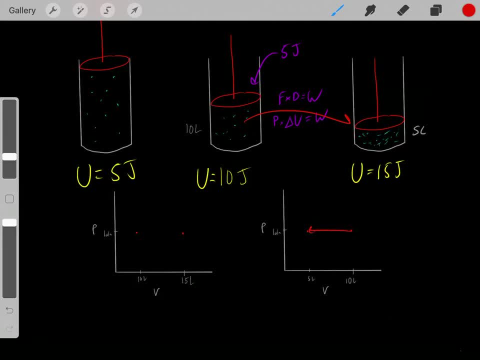 what would happen. this change would be represented by this, by a line going in this direction. We were originally here. now we're here. This original system was this. now we're here. Now we're at this final situation, And something important to note is the volume. 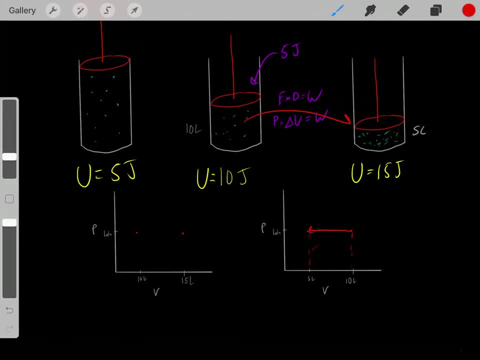 underneath these PV diagrams, this volume underneath this line, represents the work that was done. Because again we know work is pressure times, the change in volume. If we have a pressure we multiply by a change in volume. we get the work done. So again we see we have. 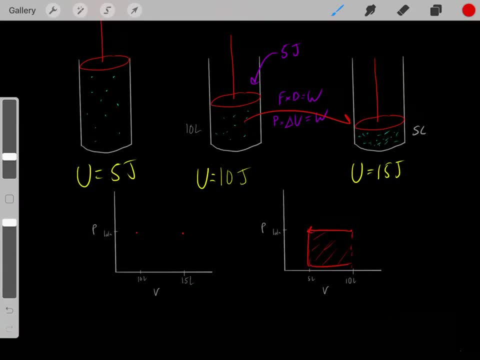 a pressure, we're multiplying it by a change in volume, And that would be this area. But something important to note, remember- when the volume is decreasing. so, therefore, when we're going in this direction and the volume is decreasing, then this is the work that was done on the gas. This 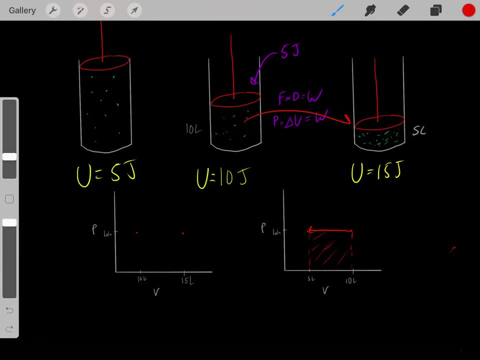 volume is the amount of work that was done on the gas, how much energy, internal energy, this gas gained. Because, again, the volume is decreasing When the volume is decreasing. so when we're going in this direction and the volume is decreasing, then we know we're compressing the gas, So we know.